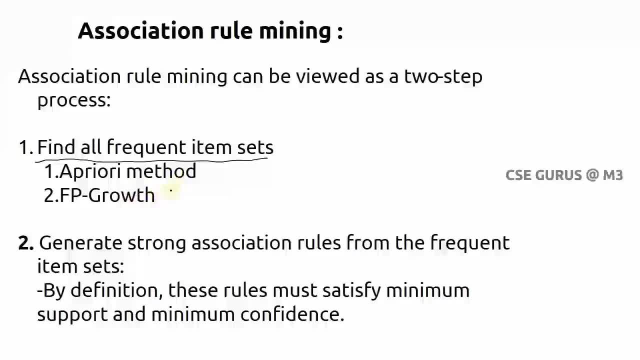 an advantage of FP growth method over a priori method. What is that advantage is? In a priori method, you are generating item sets. In that item sets. some of the item sets may not be frequent, So in order to generate all those item sets, it is definitely a complex thing. 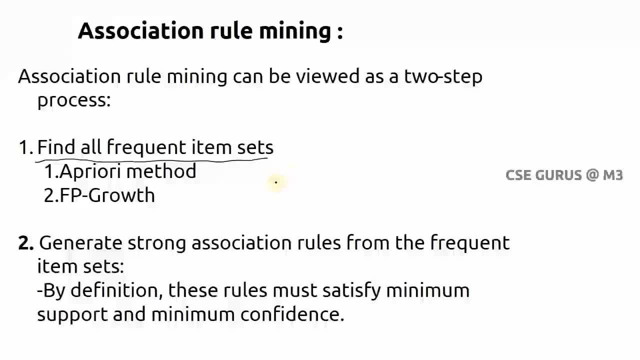 If I have more item sets in a transaction. so generating all those item sets is a complex one, In that all the item sets, most of the item sets, may not be frequent, Whereas in FP growth we are generating item sets Which are frequent only, Which are only frequent, Those item sets only we are generating. That's. 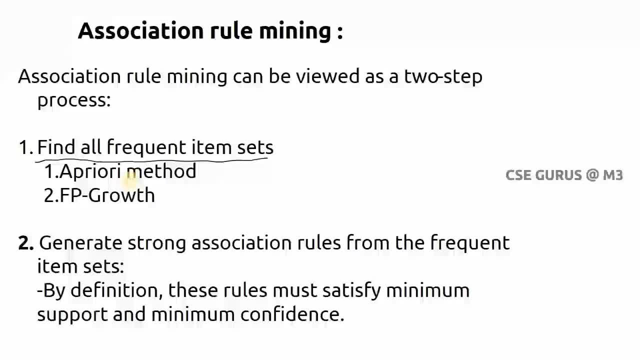 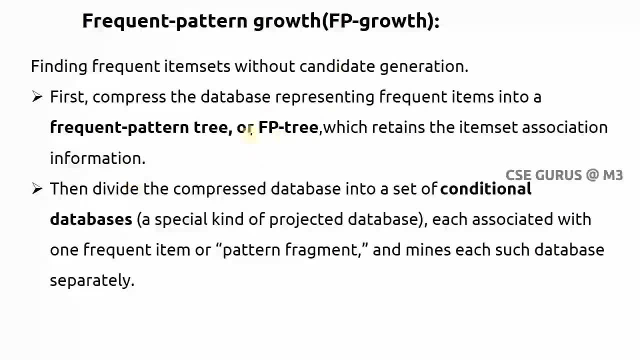 why this is a less complex compared with the priori method. So we will see here what is this FP growth method? So here you have two steps Like: first you need to construct FP tree, That is, frequent pattern tree. After that, from the frequent pattern tree, you 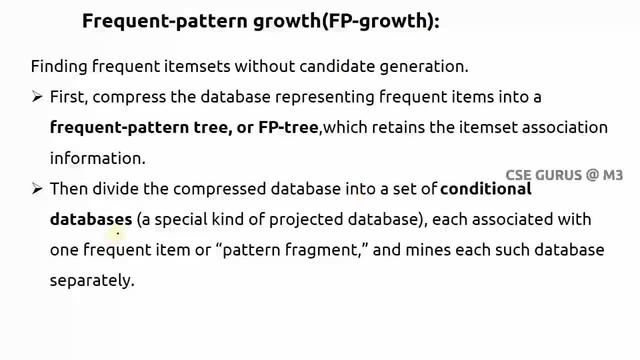 need to divide it into conditional database, Database you need to create. So anyway, we will see this one, How to construct a tree, How to make this conditional database. So we will go for step by step. So first of all, we need to: 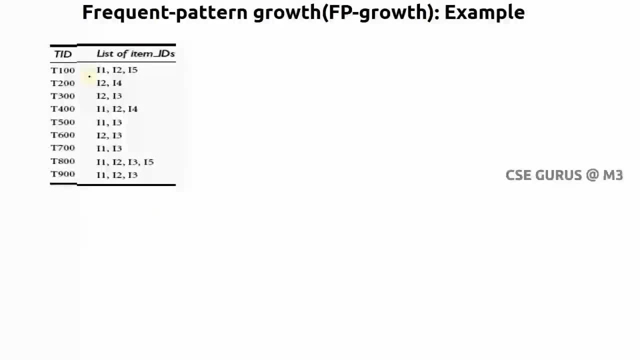 construct FP tree. Let us suppose I will consider this. one is our main transaction database where of course minimum support- I will take here minimum support- is given as 2. That is a minimum support count. So totally 9 transactions are there in each transaction. What are the list of? 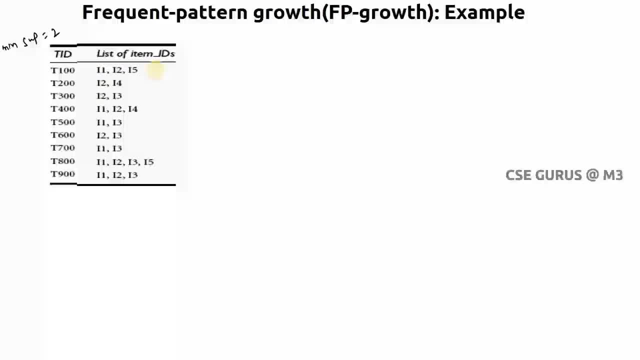 items that are purchased is given. We will consider this one, And we need to construct a FP tree first. So, like this FP tree, we need to construct. Anyway, I will explain how to construct this one. So, in the first step, what you need to do is, first you need to. 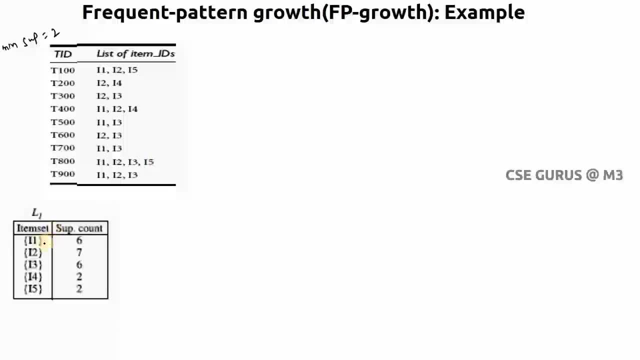 construct we need to write list of item sets with support count. So for each item set I1, what is the support count? How many transactions consisting of I1? That means 1,, 2,, 3,, 4,. 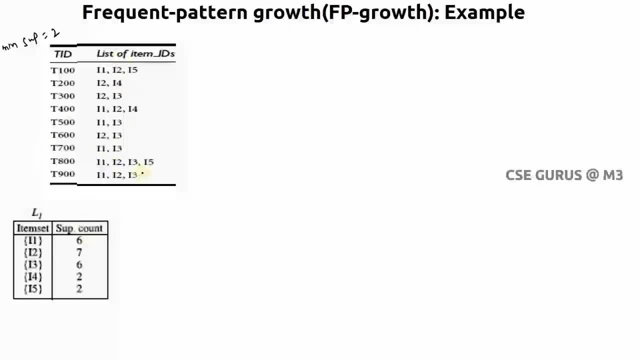 5, 6.. So that is 6. I2, 7 transactions you can see here. So like this, we need to write the support count Now. remember this point very clear. In the next step, what you need to do is you need to write these items in descending order. You need to write: 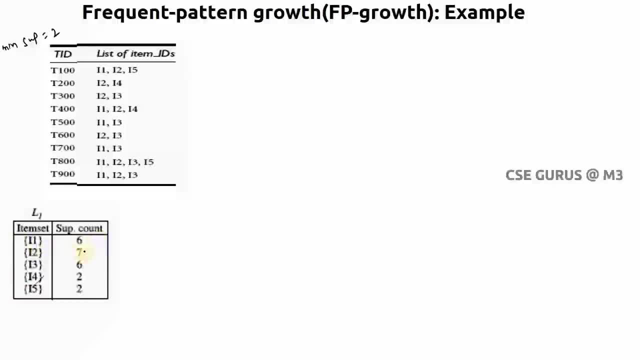 these items in descending order of their support count. So how to write this one? So, after writing into descending order, this will become like this: So where I2 has highest now, that is why first, after that, I1, I3- both are same. That is why you can take anyone. I am taking I1 first, after that. 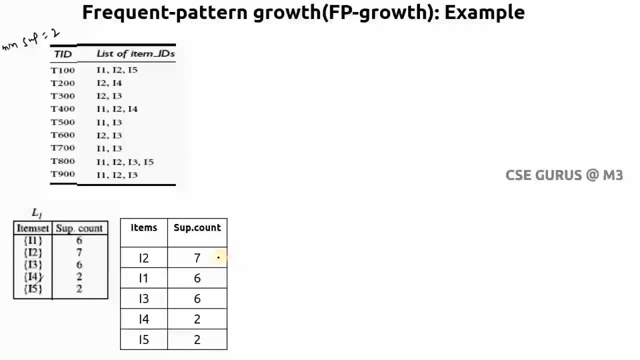 I3,, then I4,, I5, like this you need to write. so this part is very, very important. after that you need to start the fp tree by taking null as root node. so null as root node. from this, now take the first transaction. what is? 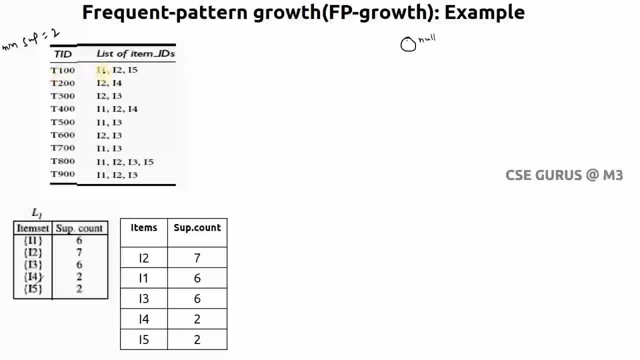 the first transaction, t100, where what are the item sets? it's consisting i1, i2, i5. so you need to consider i1, i2, i5, from that i1, i2, i5. arrange these things, these items, in descending order. in this descending order, which comes first, i2 comes first, after that i1, after that i5. so i'm writing. 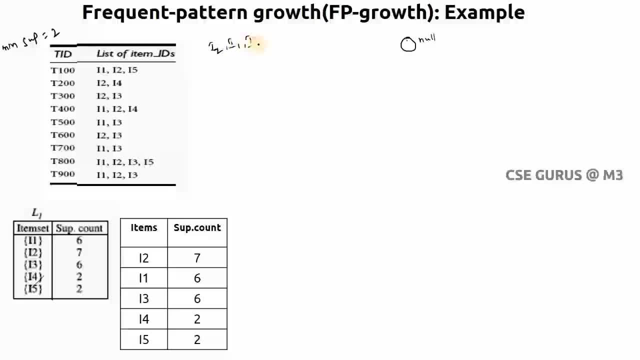 here: i2 first, then i1, next, then i5. so whatever the transaction items are there that you need to write in the descending order of their support code, so i have written: isd is i2, next i1, next i5. after that you need to start from here. i i don't have any left node. that's why i start from left. 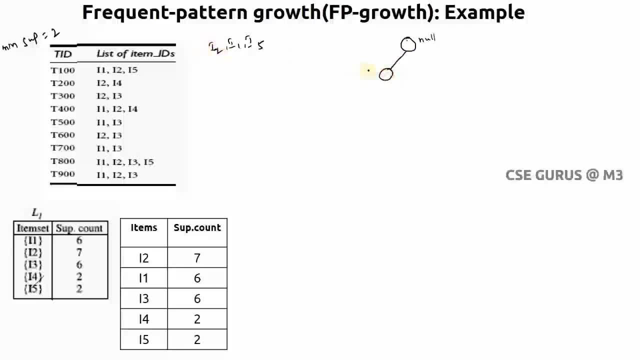 that is one node where the first item you need to consider that is i2, where the count you need to give as initially one from i2, from i2 you need to consider i1. so i'm writing i1 here from i2. i1: the initial count is one here from i1. there is next is i5. 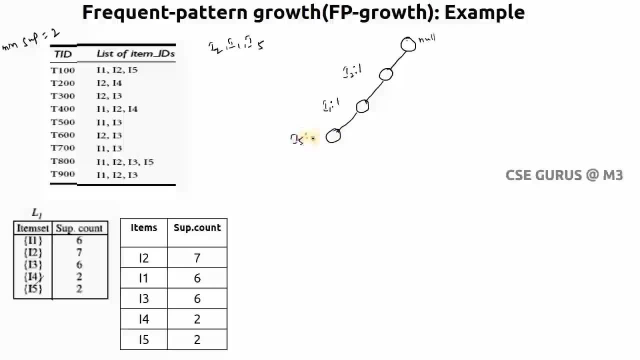 you need to take i5 next. like this: you need to write first: so i2, i1, i5. why? because i2 is the highest support count, then i1, then i5. this is the first transaction finished. next transaction: i2, i4. so if i make it into an order which will come first i2, only then i4, only because 7 is. 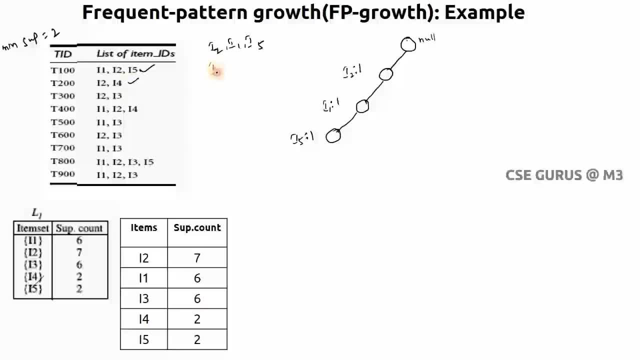 highest. so i2, i4. no need to change the order: i2, then i4. so now start from your root node. check for: is there any i2 node for this null root node directly you need to check. okay, if you have here you cannot take, you need to create another one. so if for null, if if i have i2, directly go to that. so 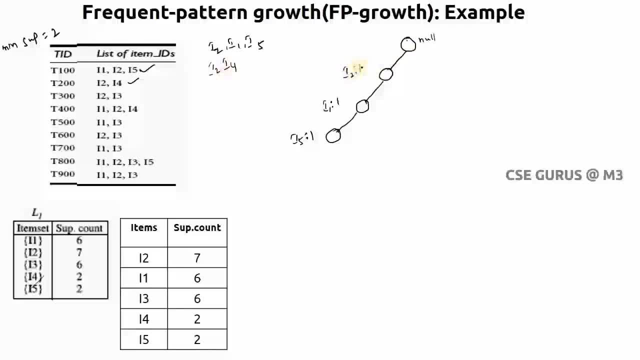 i have i2 directly. that's why i'm going here i2. that's why already count is one. now i need to make the count is two now from i2. is there any i4 from i2? i need to check. no, so i'm creating i4 here. 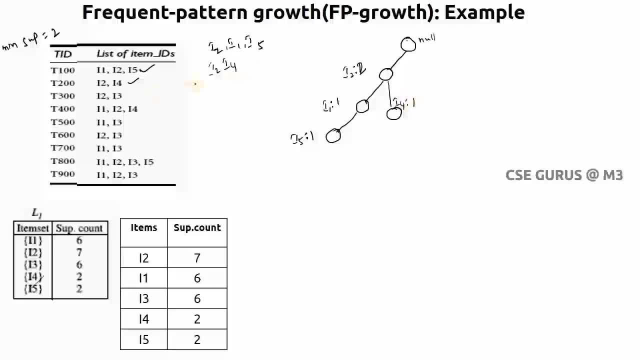 so i'm creating i4 and making count as one. now this one is over. next i2- i3. so i2- i3. first, if i make into an order, of course, the same thing: i2- i3. no need to change the order now. from root, node i2 is: 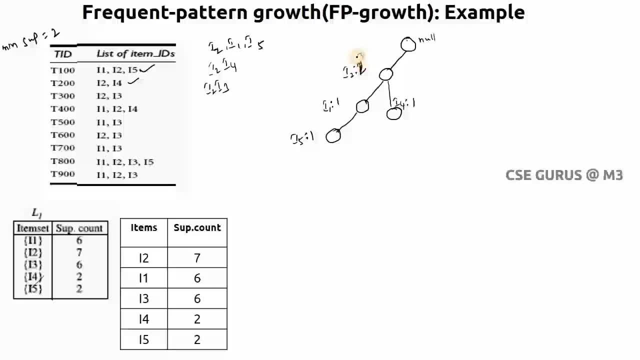 yes, so change the count. that is three now from i2. is there any i3? no, so i'll make i3 here. so i3 count is one now after this transaction: i1, i2, i4. if i make into an order it will become i2, i1, i4. why? 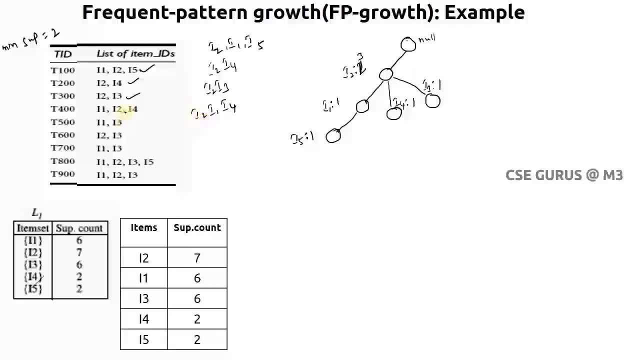 because in the descending order, so of count i2, so from root node: i2 is there, yes, so the count is four now from i2. i1 is there? from i2? i need to check. i1 is there, yes, so count is two. previously it is one, no. next. 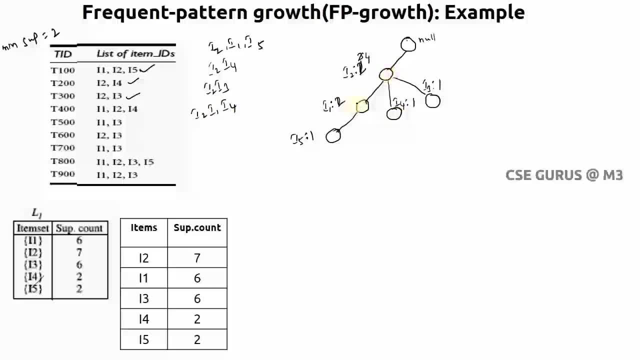 from i1: is there i4? see. from i2 it is i4. from i1: there is no i4. so i need to create i4. here the count will be one like this: you need to do next i1, i3. so if i make into an order, 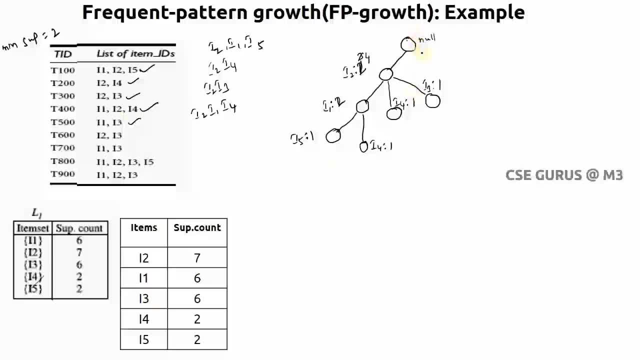 both are same, only i1, i3. so from null node, is there any i1? no, directly. i2 is there, so there is no i1 here. here it should be. i1 is here, so what you need to do is you need to generate a separate node- i1- and make that count as one. from i1 i need to take i3. so from i1, is there i3? 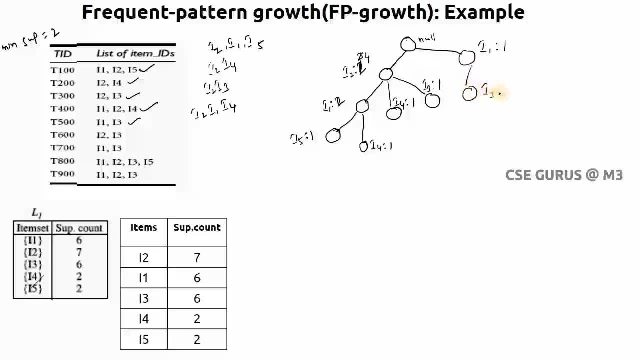 no, i need to generate i3 here, so the count is one. so this is finished now i2, i3, so i2, i3. of course it is in the order only. so from root node i2 is there. yes, count is one more from i2 is there. 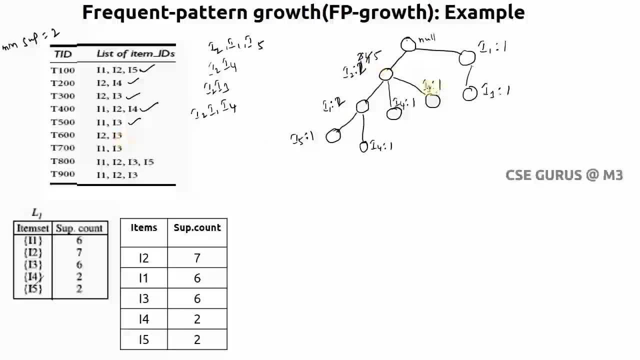 any i3 for this i am taking. is there any i3? yes, i3 is there count. i am incrementing to two. this is finished now. next one is i1, i3, i1, then i3. of course, order only. so from root node: i1 is there, yes. i3 is there, yes. from i1: i3 is there, yes, two is the count now. 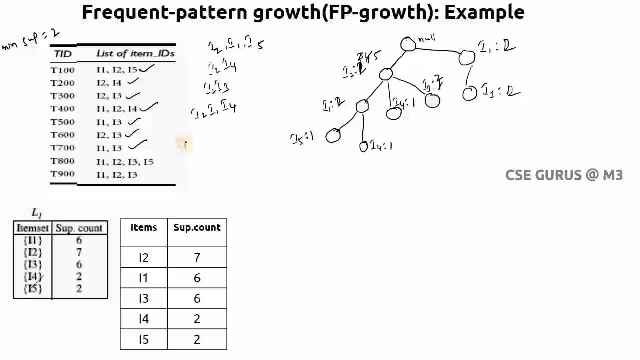 this one is finished. next i1, i2, i3, i5. if i make into an order, i2 will come first, next i1, next i3, next i5, like this: you need to write so: i2, i1, i3, i5 from root node. i need: 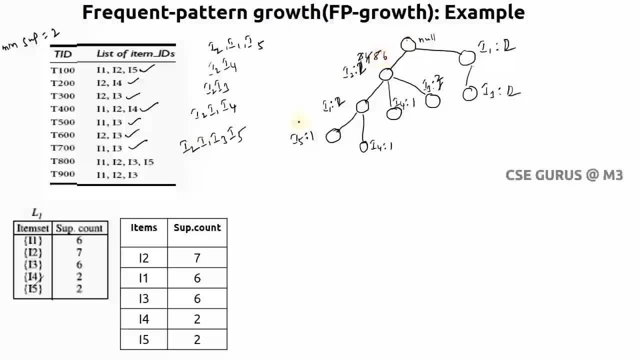 to check i2. is there? yes, now from i2: from i2: you need to check i1. is there? yes, so the count is three. now from i1: i3 is there? from i1: you need to check i3. is there no i3. so 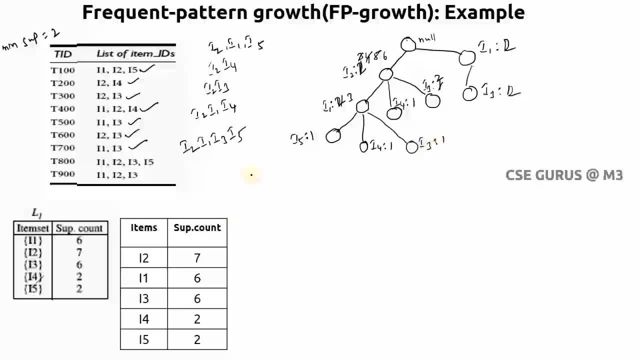 i will take here i3. the count is one now from i3, i5 is there no? so i will take i5 here. count is one like this. you need to consider now. this is finished. the last one: i1, i2, i3. if i write it to order: i2, i1, i3, so i2 from. 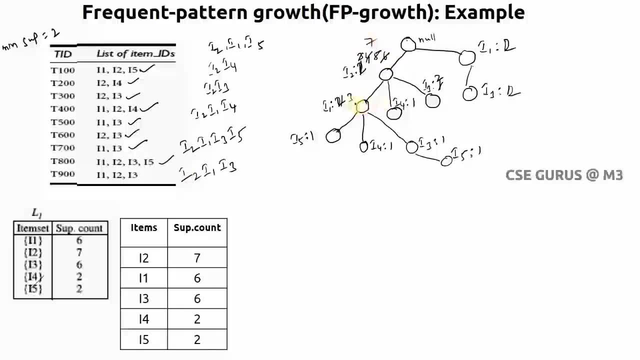 root node. i2 is there. yes, the count is seven. from here. i1 is there. yes, the count is four. now from here. i3 is there. yes, the count is two. like this you need to do for each transaction. this is we call it as fp3. you can verify it. so, for i1, if first, if 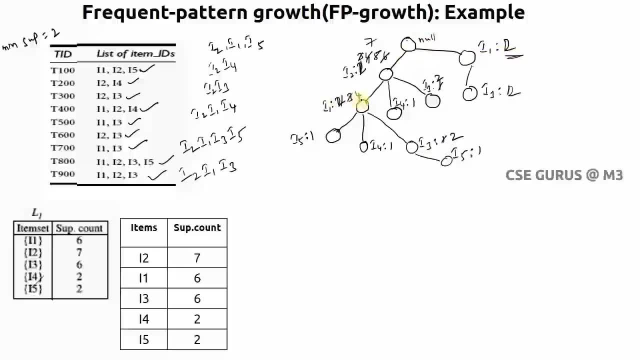 you consider i1: count is here two, here four totally six, so verified. next, i2: what is the total count? seven verified. i3: total count should be six, so here two, here two and here two totally six. and i4, that is two here one, here one, verified, and i5, two, so here one, here count is one verified. so like this we need. 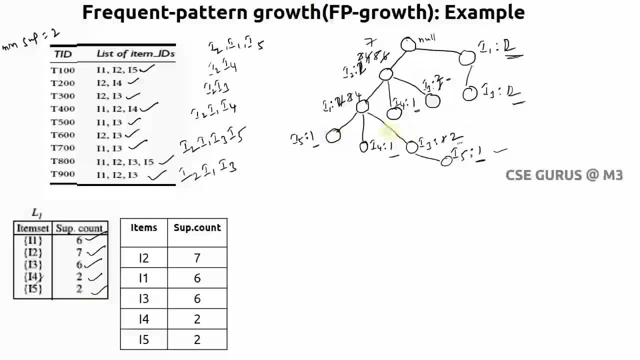 to verify whether we have done it correct or not. so this is what we can do for construction of fp tree. so this is the procedure now. this is the first step, that is, the construction of fp tree. after constructing, we need to go for conditional database. so what is that we will see here? 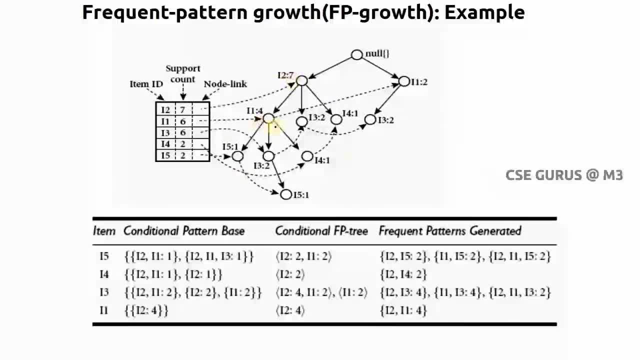 so this is what we have constructed till now: i2 count is seven. next i1, four like this. we have received everything now in the previous one. now, after that, what you need to do. so i i'll explain very easy one, this one. so you need to write a database, like having attributes, like what is. 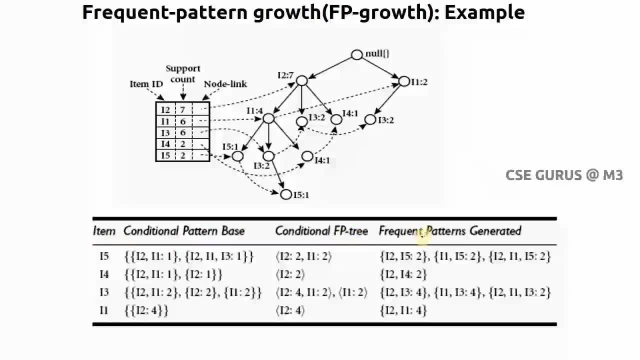 the item conditional pattern base: conditional fp3, frequent pattern generated. so how to get this one? so how to do this one from this one? so we need to consider our database. in the database check for the least support count. what is the least support count? i5, which is two in. 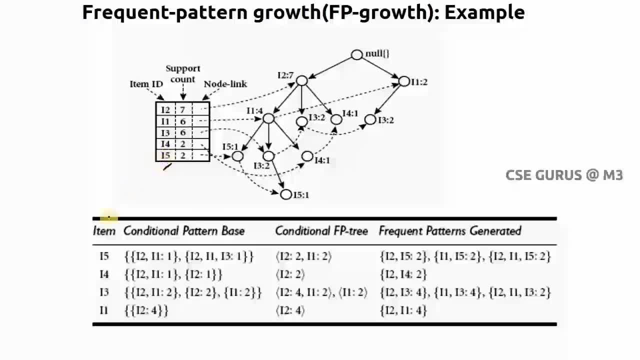 the database. of course, i4 also, you can take anyone. i'm taking i5, so i5 i need to consider first. so which is the least support count that i need to consider? now go for your fp3. where is i5? you need to check. so here is one i5, here is one i5. so how you are traversing from root node to this fp3. 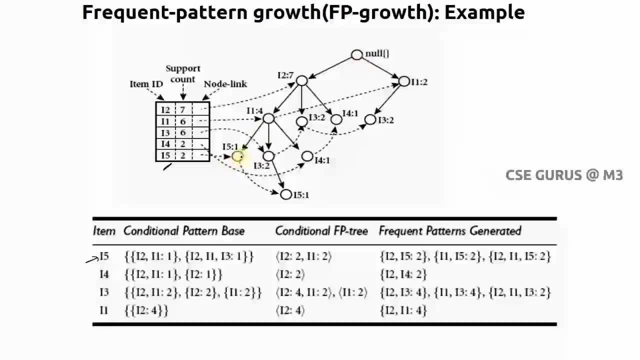 i5- how you are traversing from root node to this i5- how you are traversing: i'm coming to i2, then i1, then coming to i5. so i'm writing i2- i1. so what is the count here? one that i am writing. 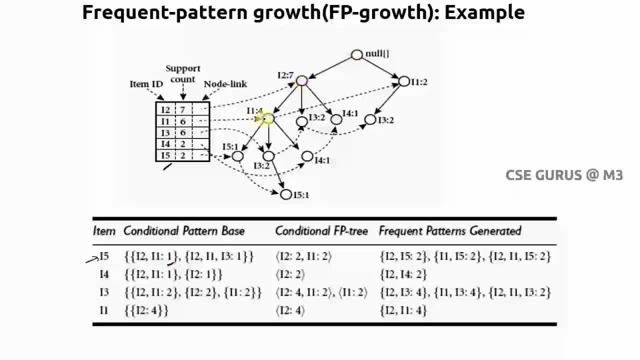 so from root node i2, i1, then coming to i5. so that's what i'm writing: i2, i1. i'm writing with the support count of this one, i5 only. i need to consider now here also one more, i5. so what is the support count? one now how you are reaching to this one from root node. 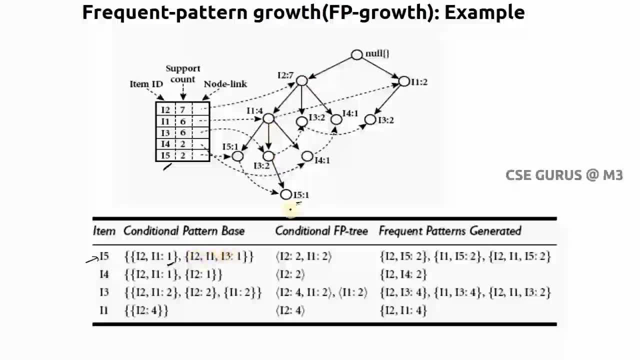 i2, i1, i3. so i2- i1- i3. what is the count one? i need to write like this: how you are traversing to the node that you need to consider now, after taking, you need to count i2- i1. that is the count. 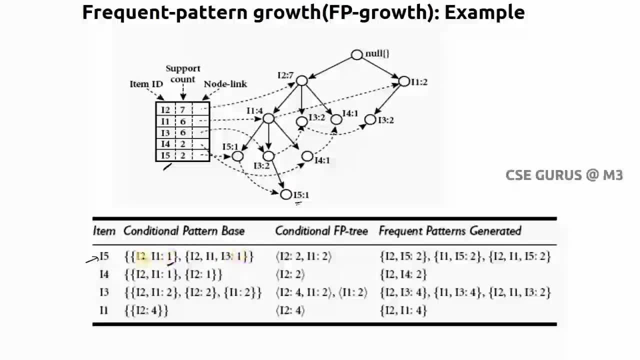 is one. i2, i1, i3- that is the count- is one. that means for each item the count is one. for i2 it is one, i1 is one. here also, i2 is one, i1 is one, i3 is one. like this, if i consider: 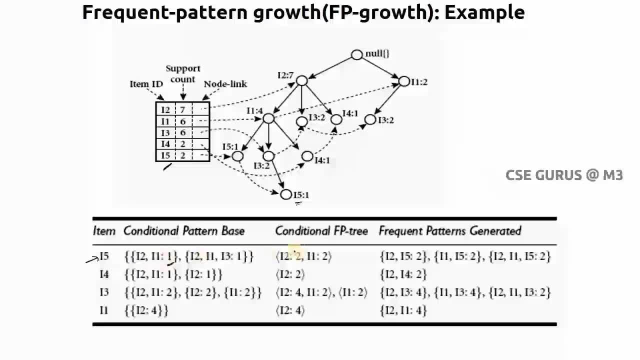 what is the total count of i2 here? one here one. totally two for i1 here, one, here also one. the count is two for i3. what is the count here? only one, no, so that's why only one is the count. why i am not writing here is: what is our minimum support? that is equals to two, no, in our example. 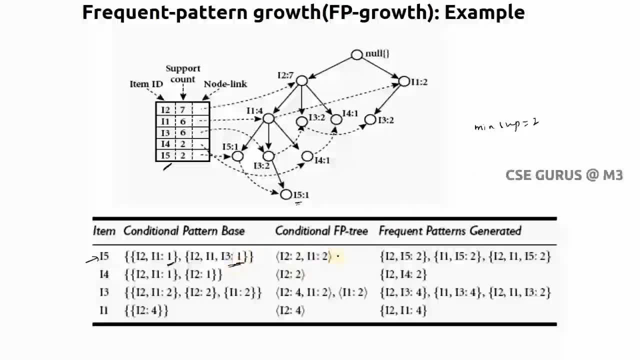 it is given. so it is not satisfying that constraint. that's why i3 will not consider here, why only i2. i have taken our i1 which are satisfying the minimum support. so like this we need to remove which are not satisfying the constraint. now, after getting 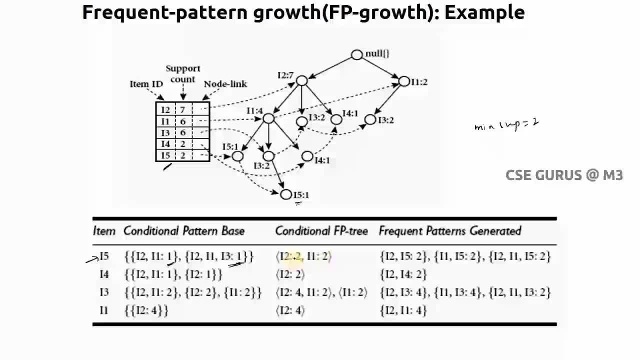 conditional fp3. you need to make this item sets. you need to join with the your source item. that is i5. so how i can make joints with i5 with i2, i1 like i2 with i5, that is the first one. i1 with i5, that is the second one. i2, i1 with i5, that is the third one like this. we need to consider. 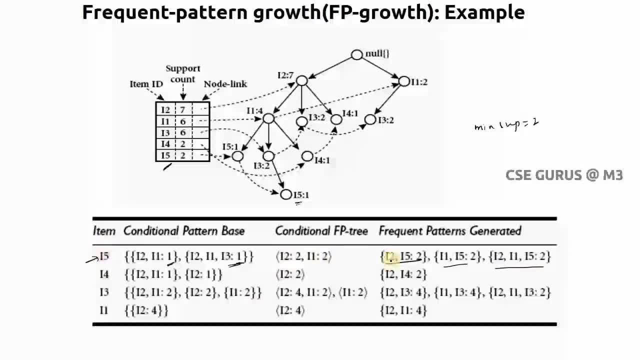 so, whatever we are getting, i'm making joints with the source item. that's why i2, i5- i made it now. so what is the count? here we are getting for i2 two. that's why i need to write here for i1: what is the count i? 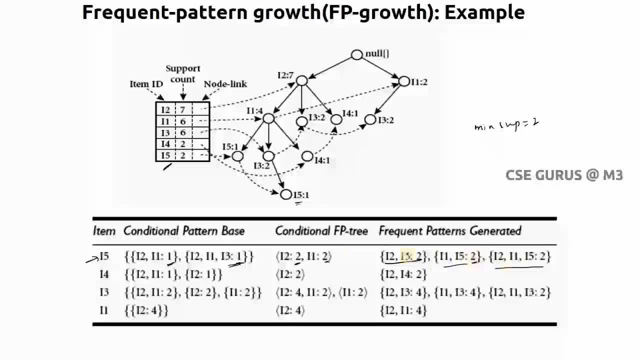 am getting two. so that's why i1 is two. now for this one you need to check i2, i1. both are there. you need to check the count two and two. so you need to if. if both are same, you need to write the count here. if both are not same, let us suppose here you have four, here you have two. 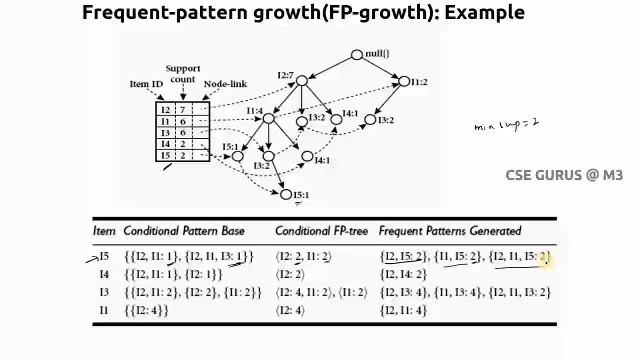 you need to take the minimum one, which is the minimum that count. you need to write here so all are satisfying the minimum support constraints, of course. we are taking only which are satisfying. that's why we'll get the same thing here. now, the next least one: i4. 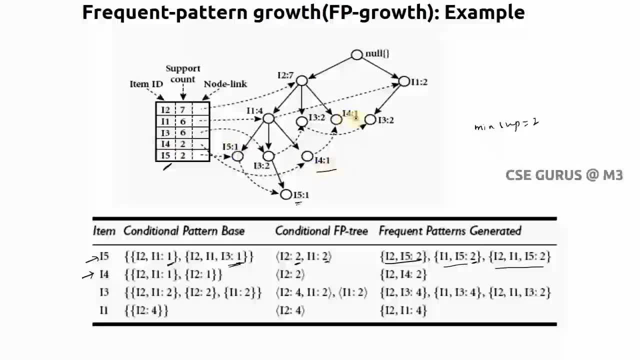 so if you go for i4, where is i4 here here now, how i am reaching to i4 here from root node. i am coming to i2, then i am coming to i4, so only i2. i am taking for this one. what is count one i am writing now, what about this one? why i am reaching to this one from root node. 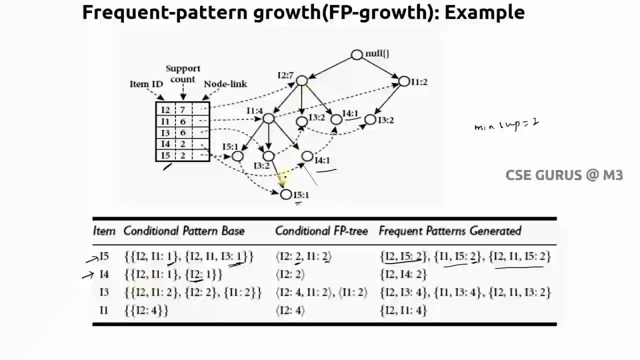 i2, i1, i4, so i2, i1, so i2, i1. the count is one here, so that i have written here. so now, after that conditional fp3, what i need to do. i2 count is one. here also, i2 count is one. total i2 is two. 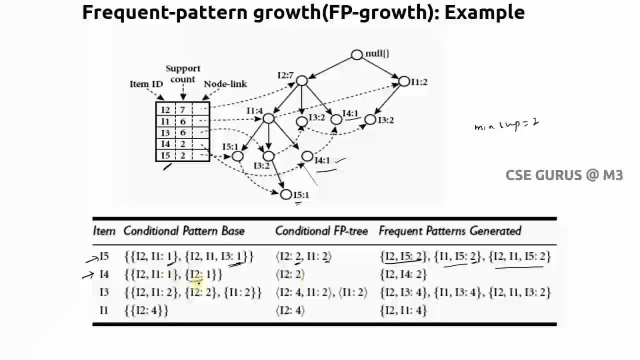 for i1 count is only one here, so one which is not satisfying. that's why i am not writing this i1 here. now what i need to do: make joins with source i4. join with i2. only one join, you will get i2. i4 with the count is two. now what is the next one? i3. so if i consider i3, so where i3 is, there you. 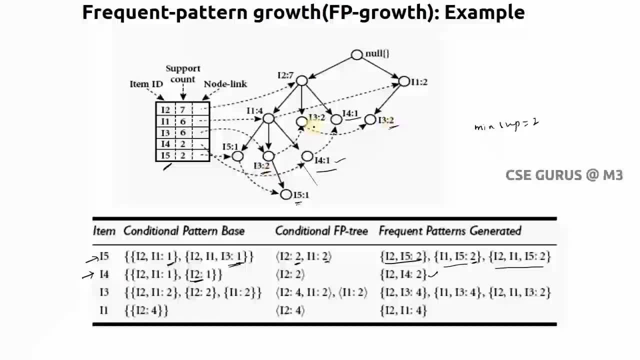 check it here: i3 is there with two count here. i3 is there with two count here. i3 is there with two count. now, first we'll go for this one, how i am reaching to i3 from root, so i2, then i1, so i have. 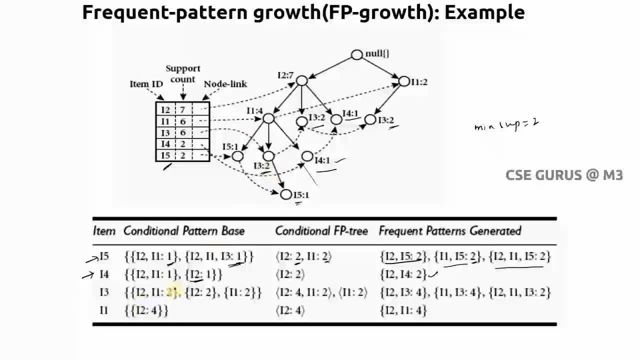 written i2, then i1. what is the count here two? that's why i have written here two count and here one i2, this i3, so i2, then i3 directly. so that's why i have written here i2. now here how i am. 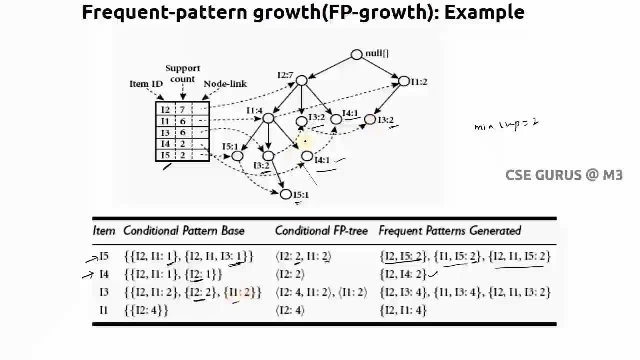 reaching i1, then i3, so i1. i have written so with the counts. whatever the counts we have writing here here, listen carefully, remember this point here here: whatever the for i3, whatever the items we are getting, not only one side, it is on left hand side as well as right hand side. 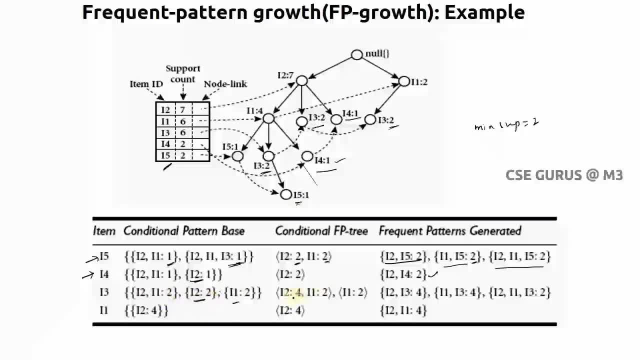 so you can see: here: i2 count here 2, here also 2, so totally 4. i have written: i1 count here 2, here also 2, i1 totally 4, but i am not including both. why? because one i1 which i have received, received from left subtree. 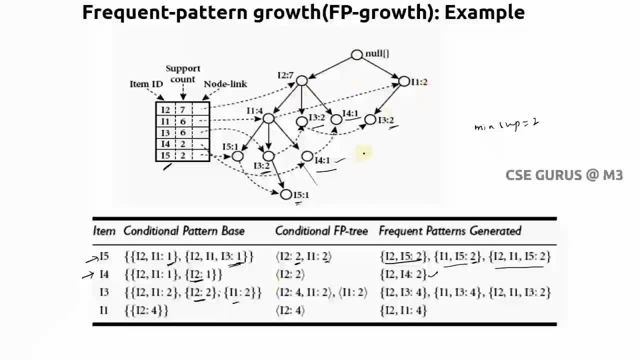 and the another, i1, i have received from right side subtree. so remember this point: one i1- this one, i have received from left subtree, this one i have received from right subtree. that's why i am not including here. that is a part you need to consider. so after this, of course 3 are satisfying. 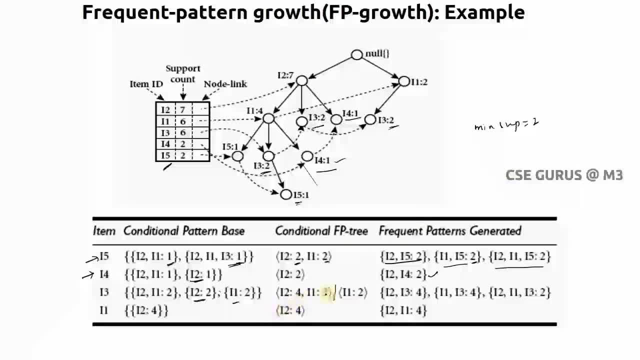 minimum support constraint, that is, count is 2. after that, if you want to make join, make these joins with i3 separately, make this join, i1 with separately. so if i make i2, i3, one join, the count is 4: i1, i3, one more join, of course the count is 2, and next i2, i1, i3. 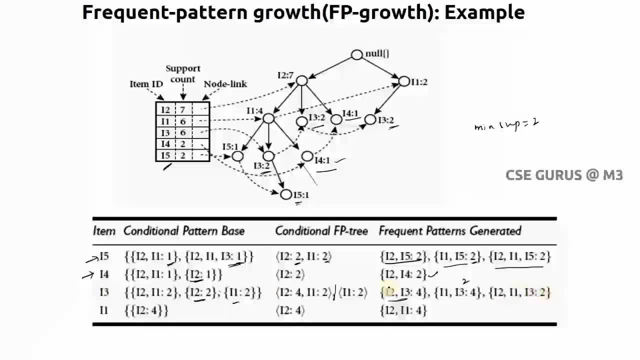 of course i2, i1, i3, one more join, and the count here four, year two. i told you know. so, whichever, the minimum two so that i have rating here. now, if i make this one, i1, i3, join, so that is two, see i1. 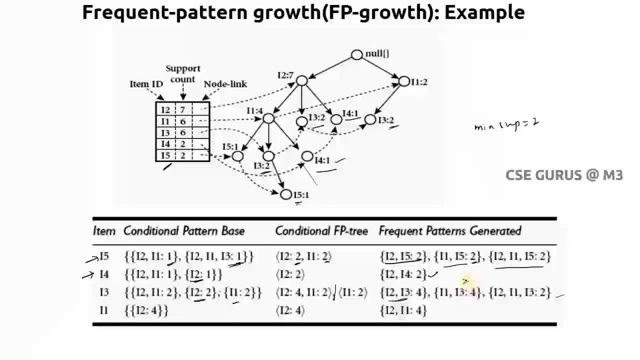 i3 join already here. it's there with two count. now again i1- i3. so totally four count. you need to combine here here you no need to combine here you need to combine. so that's what i1- i3 is four. why? because i1 combination with i3, here two, i1- i3 combination here with two. that is left subtree. 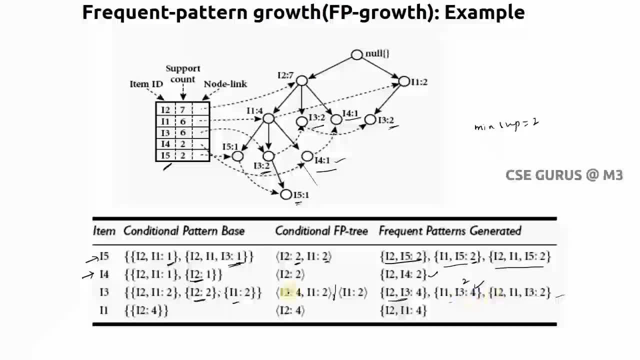 and right subtree. i am combining. that's why i1, i3, now four. like this you need to generate. now, coming to the next one: i1. so where is i1 here? four, here two. so how you are reaching to this i1 from root node by i2, so i2. i have written with this count four and here there is no in between. 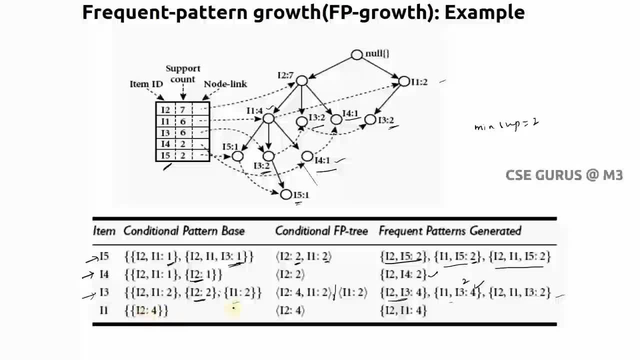 node. that's why nothing you need to write. so i2 four, i2 satisfying. that's why i'm writing combination i2 with i1 four. i've written here and coming to the last one, i2, anyway, i2 here, totally seven. there is no in between. you won't. 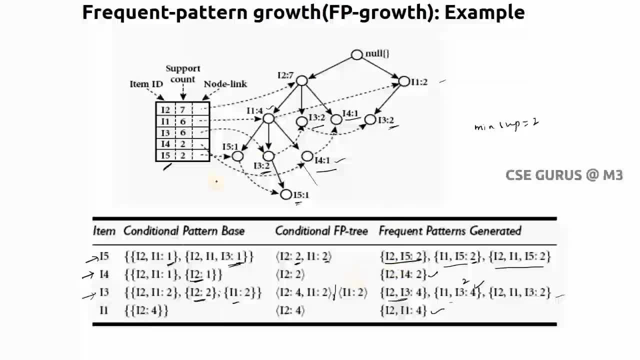 find that one. so, like this, you need to generate and where is our answer why you are doing all those things? for because of getting frequent item sets. so all these things here, whatever you are receiving, all these things are frequent item sets. you can observe so three frequent item sets: i1, i2, i5, i1, i2, i3. so these two are three frequent item sets and these 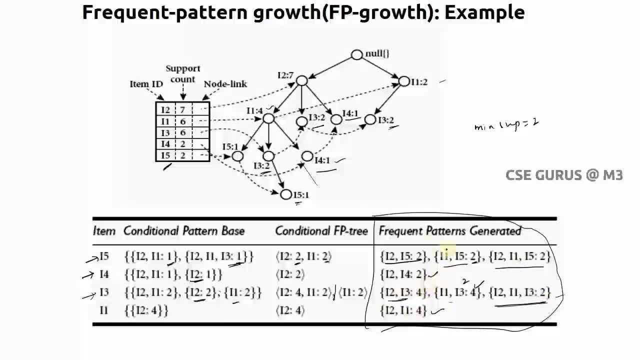 are two frequent item sets. if you compare with apriori algorithms here in fp growth, i generated only those sets which are satisfying our constants. i have not generated here like i2, i5, i2, i5, which is not frequent like this, so only frequent. i am generating which is less complex compared to the 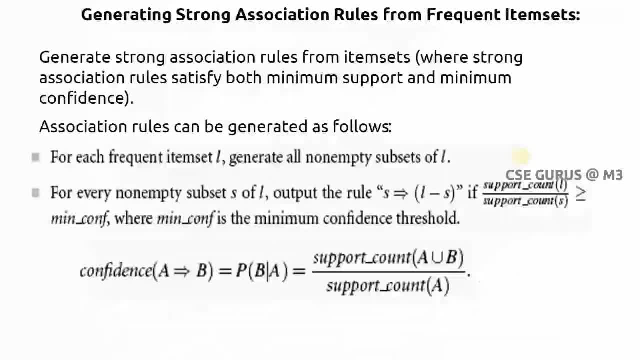 algorithm. so this is about fp growth method. now, after getting frequent item sets, we'll go for generating strong association rules from frequent item sets. so how to do this one? so those which are strong association rules, those rules must satisfy both minimum support and minimum confidence. anyway, that minimum support we have done in the previous one, that is, with apriori algorithm. we have checked. 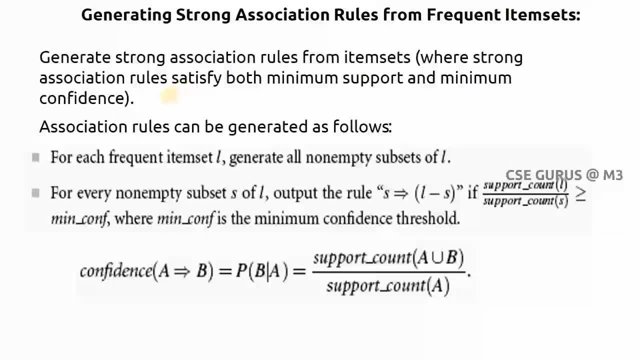 for every item sets with minimum support count. now the constraint with minimum confidence will come here, so we'll see that one. so how to do this one? it's a process. association rules can be generated as follows: the first step, anyway, we'll do here and here you require how to find the confidence. also, this is the formula for confidence: a implies, b is. 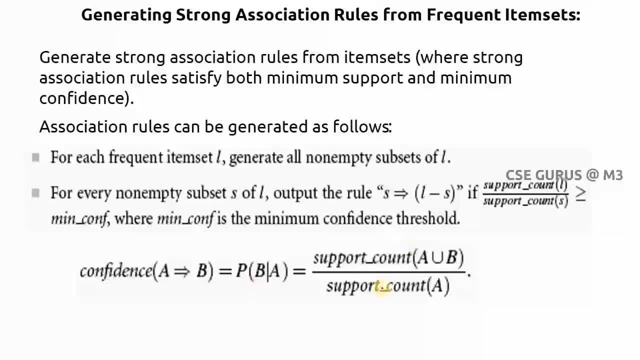 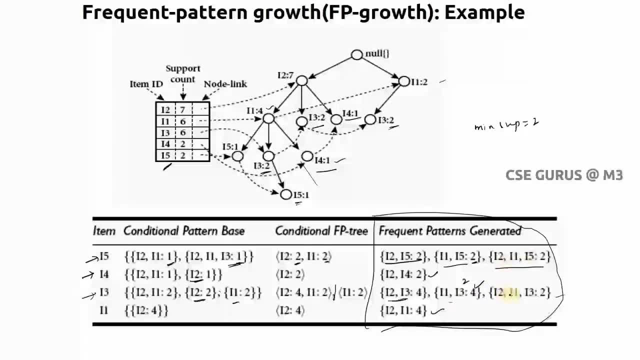 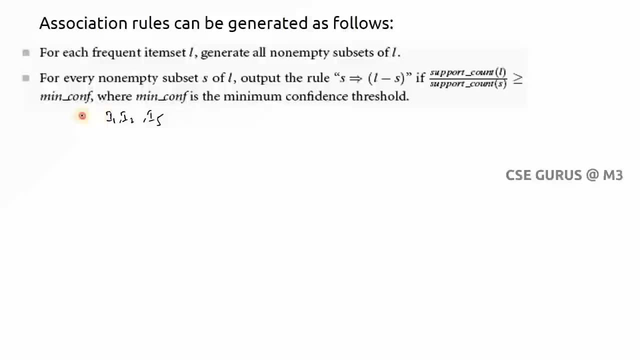 the one rule for that: support count of a, union b by support count of a. we'll see this one now how to generate. so three frequent item sets: i1, i2, i5, i1, i2, i3. so i'll take i1, i2, i5 for each frequent item set. so i have taken l, which is frequent item set, that is, l. 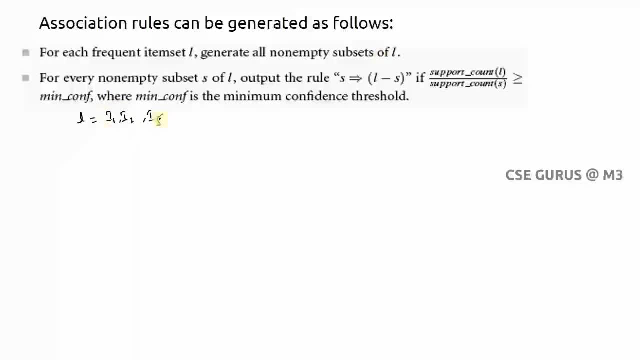 generate all non-empty subsets of l. so what are the non-empty subsets of i1, i2, i5, if it? if this is a one set, what are the non-empty subsets? so all subsets i am writing here. so empty set we are not supposed to take after that. i1 is a one subset, i2 is another, i5 is another. then i'll go for i1. 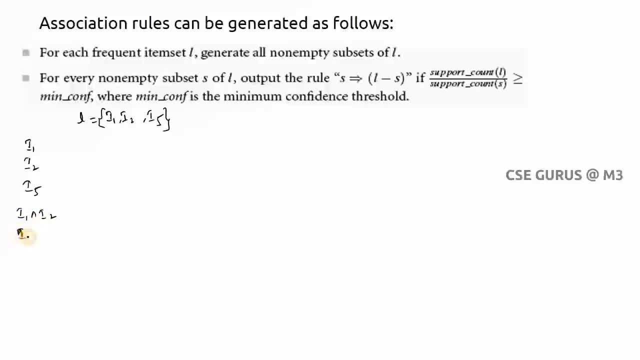 then i'll go for i1 and i5, then i'll go for i2 and i5, then i'll take i1 and i2 and i5. so all these are non-empty subsets of i1, i2, i5 i've taken. so after that, for every non-empty subset of s. 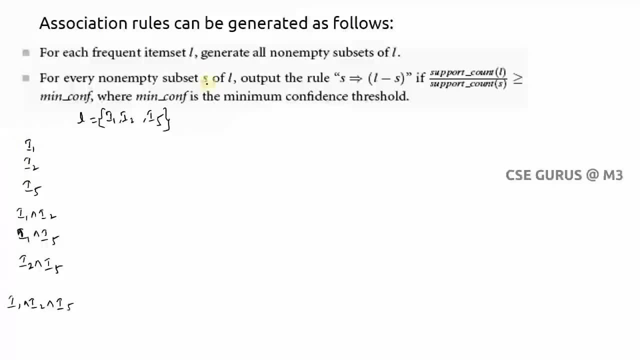 so each one. i call it as yes. so each subset i'll represent with s of l output, the rule. what he is saying is we need to write a rule that is: s implies l minus s, so i1. if i1 is s, what is l minus s? l means all these things, so l minus i1, so remaining three. 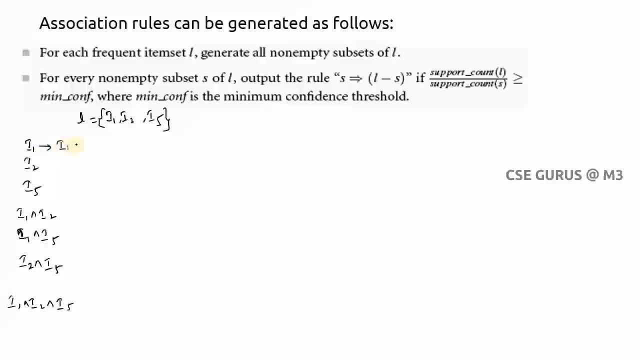 two will come here. so i1 implies i2 and i5. here i2 implies i1 and i5. i5 implies i5. here i1 and i2. see s is i1 and i2. what about l i1, i2, i5, if i make minus? 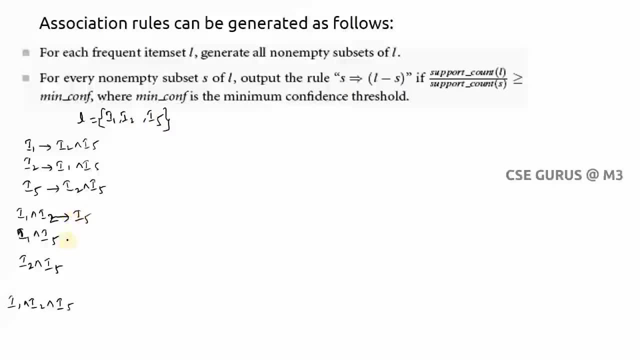 and the right hand side, i'll get only i5. so here i1, i5. that's why i'll get only i2. here i2, i5. i'll get only i1. so here all those things are there, l minus s, both are same, so i'll get pi here. 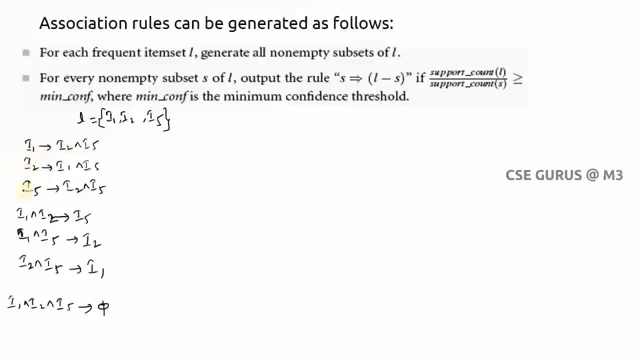 so if i observe those rules, left hand side, right hand side is there for every rule except this one. there is no, so that's why we'll neglect this one and we'll take these six rules only first. so we generated rules first among these, which are strong association rules. how to find it so? for that we 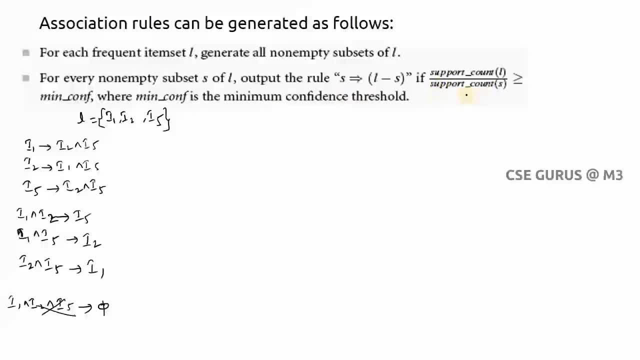 have a constraint where which one. you call it as if support count of l by support count of s is greater than or, of course this is, we call it as confidence. the formula for confidence is greater than or equals to minimum confidence. so first of all, we'll find confidence value for each one. 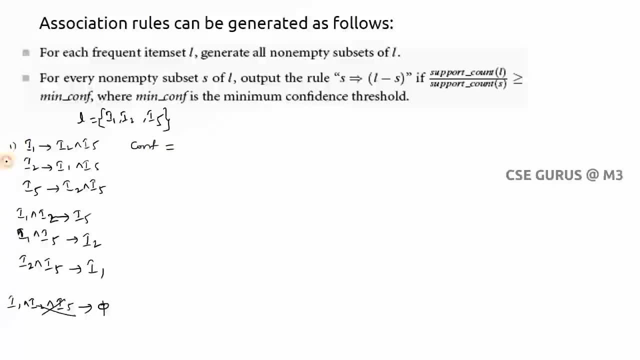 so confidence value for the first rule. so there's a rule one, two, three, four, five, six. so confidence is equals to support count of l by support count of s. what is l? i1, i2, i5? so what is the support count of i1, i2, i5? if you see in our previous one, in frequent item sets you can. 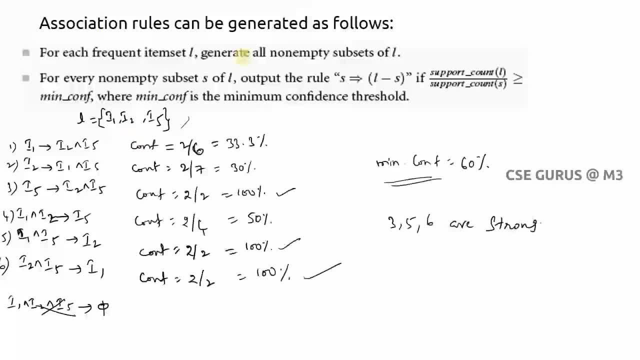 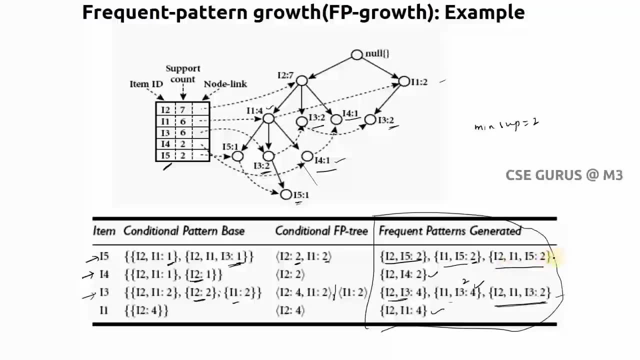 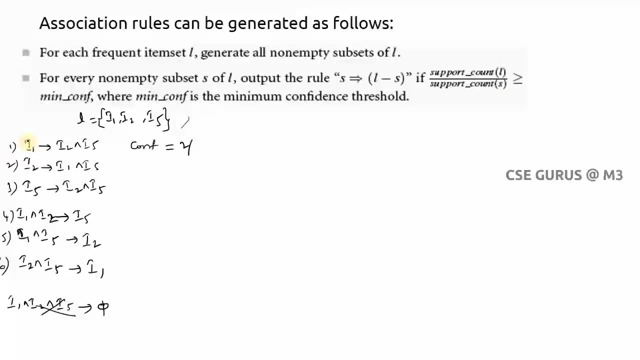 observe what is the support count of i1, i2 and i5, which is given in p growth. so i1, i2, i5. you can see here i1, i2, i5, the count is two. support count of s s means left hand side, that is i1. so what is the support count of i1? so the support count of i1 is: 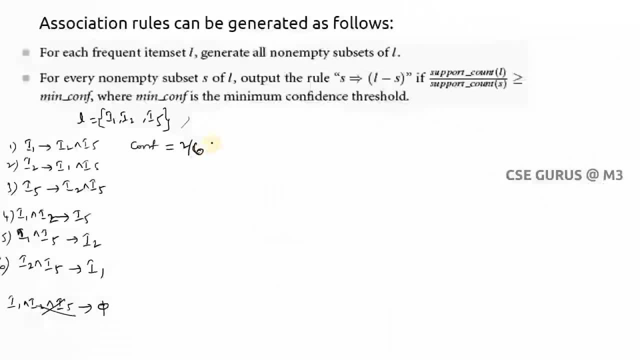 six here like this we need to consider. so two by six, which is approximately 33.3 percentage. next, if you go with the next one, confidence, that is, support count of l by s, l means, of course, two only by support count of what is s value left hand. 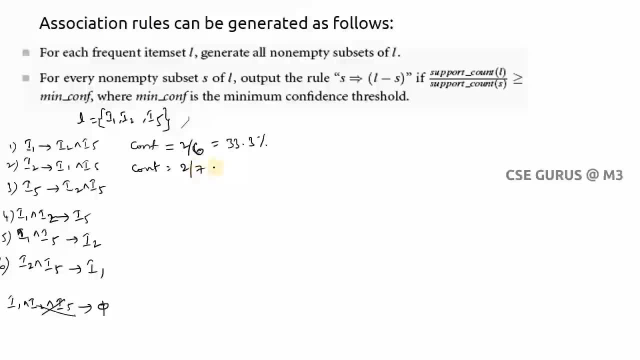 side, that is i2. what is the support count of i2 seven? you can observe there, you can see in that. so this is approximately 30 percent. i'm taking approximately. confidence is equals to. next: support count of l: l means two by what is on the left hand side, i5. 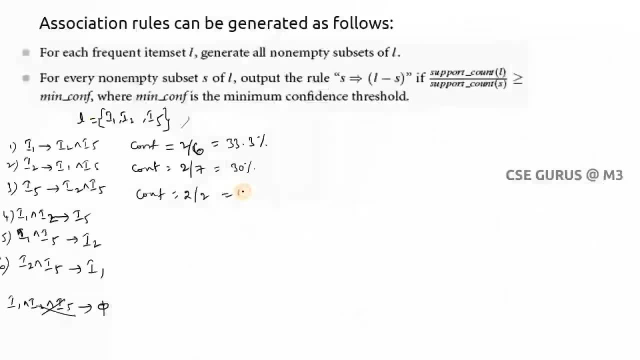 what is the support count of i5? so that is two only so, which is hundred percent. next, confidence is equals to here. support count of l means two by what is on the left hand side, i1 and i2. we need to check for support count of i1 and i2. 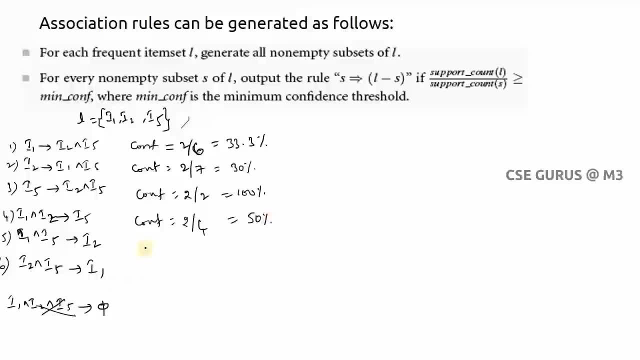 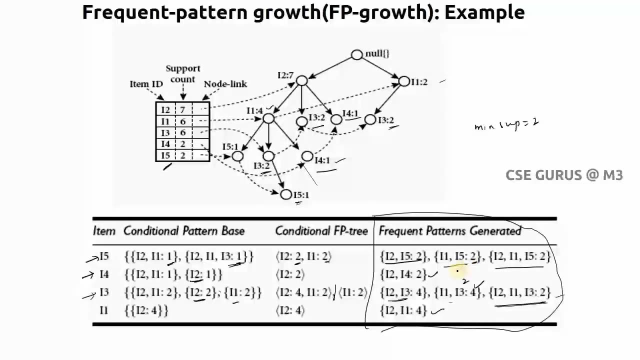 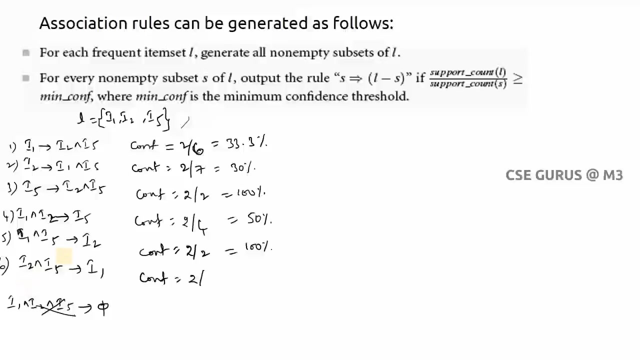 so which is one by two, which is fifty percent. next, confidence is equals, so two by so what is there? on the left hand side? we need to check i1 and i5. what is the support count of i1 and i5? that is two hundred percent. and the last one support count of l means two by i2 and i5.